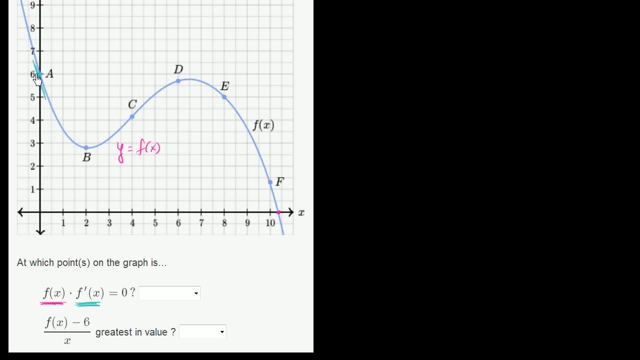 is going to be some negative value. It's the slope of the tangent line. Similarly, f prime of x when x is equal to 4, that's what's going on right over here. that's going to be the slope of the tangent line. 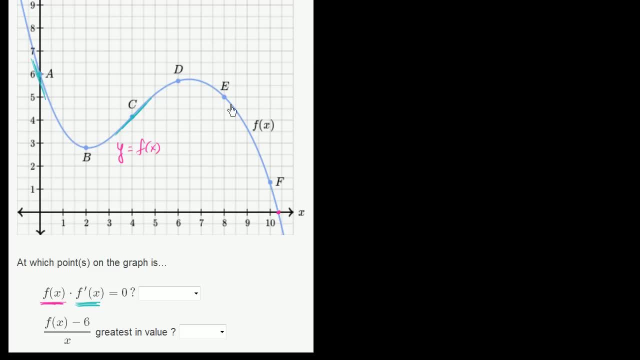 It's going to be a positive value. So, if you look at all of these, where is the slope of the tangent line 0?? And what does a 0 slope look like? Well, it looks like a horizontal line. So where is the slope of the tangent line here? horizontal. 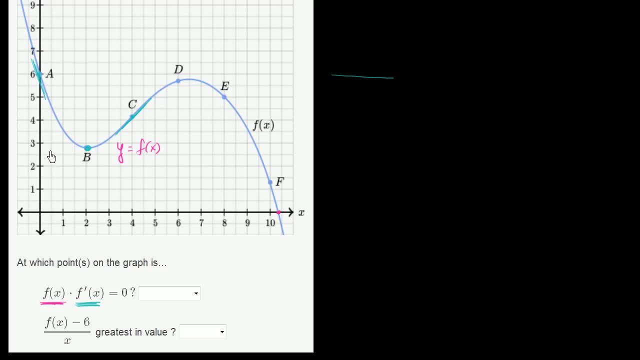 Well, the only one that jumps out at me is point b. right over here It looks like the slope of the tangent line would indeed be horizontal right over here, Or another way you could think of it is the instantaneous rate of change right of the function. 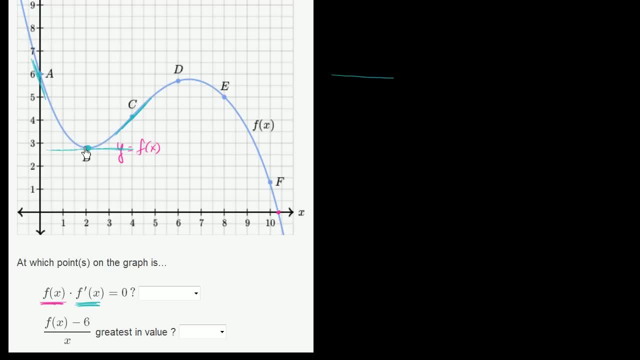 right at x. So if x equals 2, it looks like it's pretty close to 0.. So out of all the choices here, I would say only b looks like the derivative at x equals 2.. Or the slope of the tangent line. at b it looks like it's 0.. 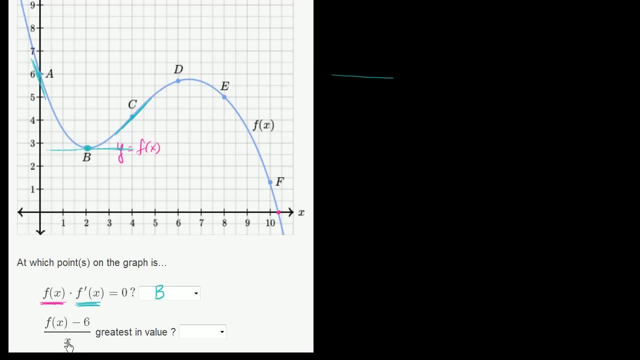 So I'll say b right over here. And then they have this kind of crazy wacky expression here: f of x minus 6 over x. what is that greatest in value? And we have to interpret, We have to think about what does f of x minus 6 over x. 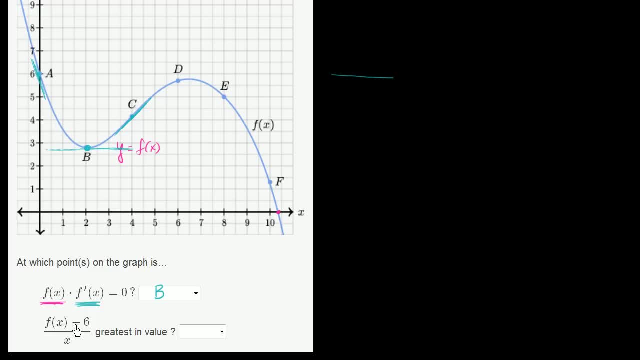 actually mean. And whenever I see expressions like this, especially if I'm taking a differential calculus class, I would say, well, this looks kind of like finding the slope of a secant line, Whenever, in fact, all of what we know about derivatives 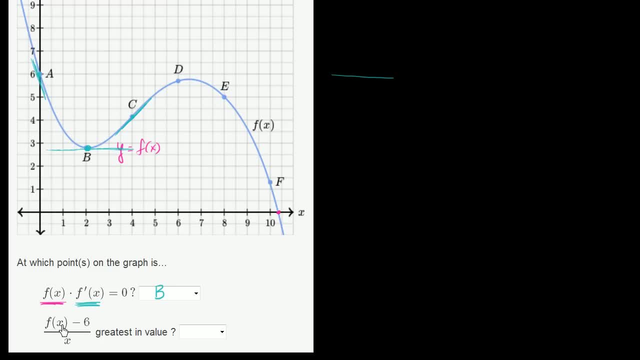 is finding the limiting value of the slope of a secant line, And this looks kind of like that, especially if at some point my y value is a 6 here, then this could be the change in y values. So I'm going to look at this. 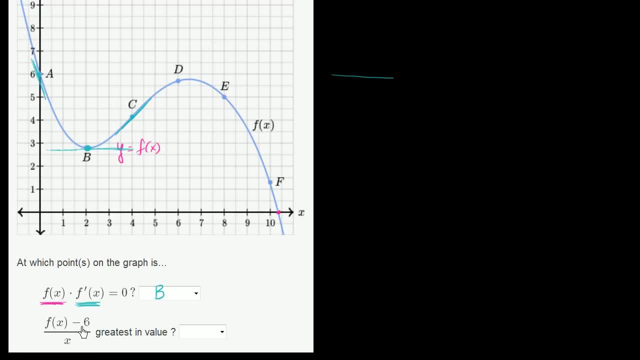 I'm going to look at this value, And if the corresponding x value is 0, then this would be f of x minus 6 over x minus 0. So do I have 0, 6 on this curve here? Well sure. 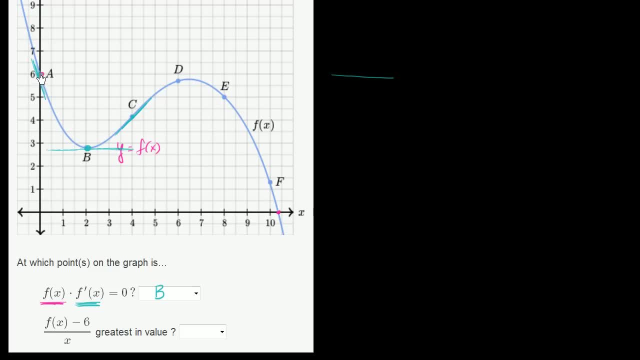 When x is equal to 0,, we see that f of x is equal to 6.. So what? this is right over here. let me rewrite this. This we could rewrite as f of x minus 6.. Over x minus 0.. 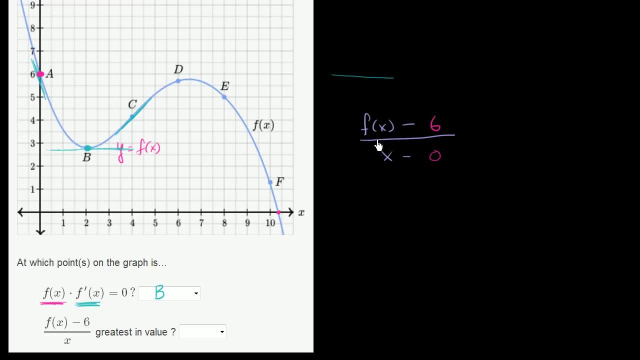 So what is this? What does this represent? Well, this is equal to the slope of the secant line between the points, between the points x and y. And what does this represent? x, f of x and whatever the corresponding f of x is. 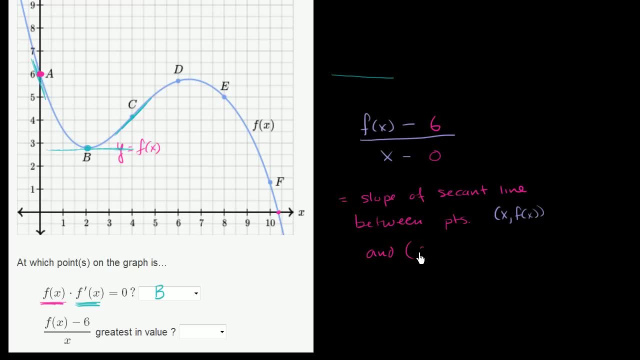 And we could write it as 0,, f of 0, because we see f of 0 is equal to 6.. This right over here is f of 0. In fact, let me just write that as 6 and the point 0,, 6.. 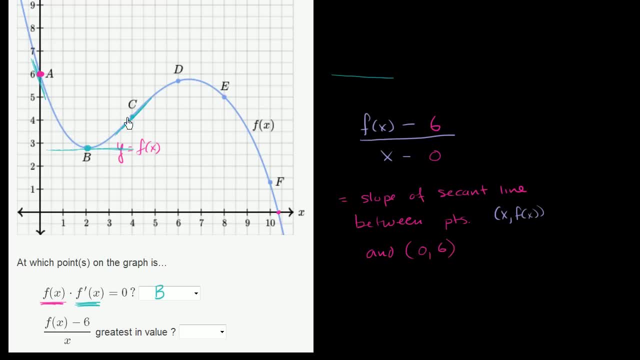 So let's go through each of these points and think about what the slope of the secant line between those points are and point a. This is essentially the slope of the secant line between some point x, f of x and, essentially, point a. 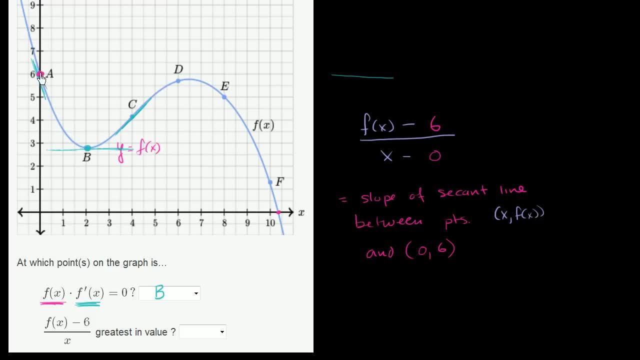 So let's draw this out. So between a and b you have a fairly negative slope. Remember, we want to find the largest slope, So here it's fairly negative. Between a and c, it's less negative. Between a and d it's even less negative. 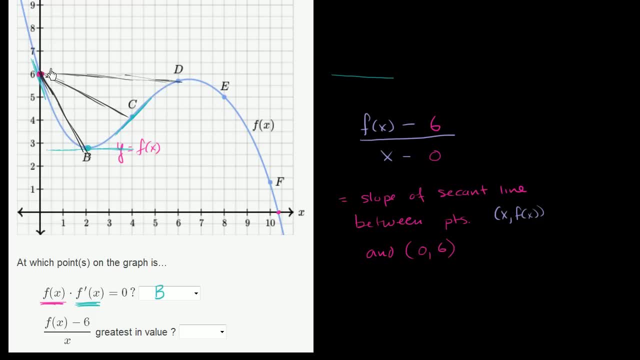 It's still negative, but it's less negative. And then, between a and e, it becomes more negative now, And then between a and f, it becomes even more negative. So when is the slope of the secant line between one of these points and a the greatest? 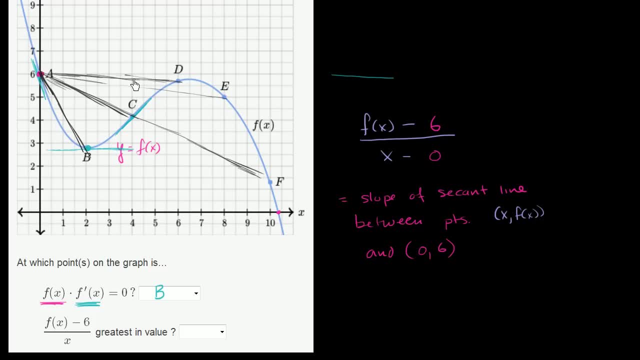 Or I guess we could say the least negative, because it seems like they're always negative. It would be between point d and a. So when is this greatest in value? Well, when we're looking at point d, At point d, x is equal to 6, and it looks like f of x. 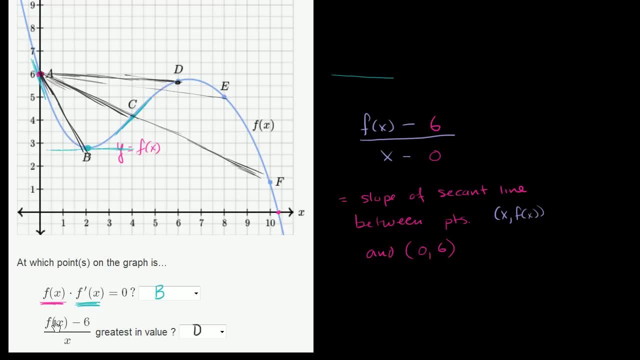 is like 5 and 1 half or something, So this will turn into f of 6, which is 5 and 1 half, or maybe it's even less than that: 5 and 1 third or something minus 6, over 6 minus 0.. 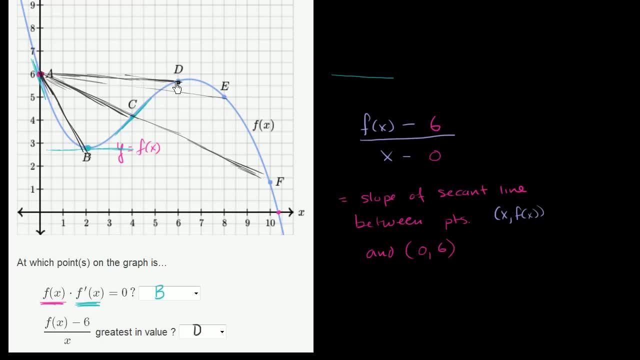 That's how we'll maximize this value. This is the least negative slope of the secant line. All right.